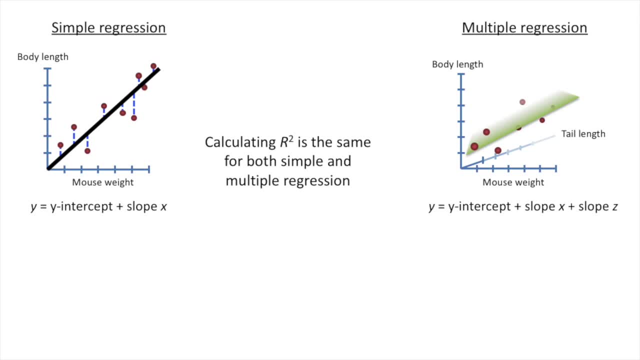 regression and multiple regression. There's absolutely no difference. Here's the equation for r-squared, and we plug in the values for the sums of squares around the fit, and then we plug in the sums of squares around the mean value for the body length, Regardless of how much additional. 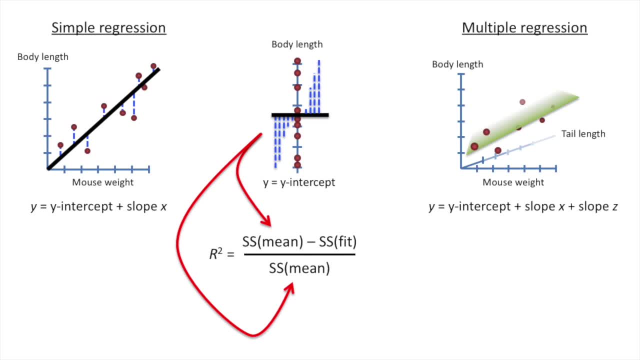 data we add to our fancy equation. if we're using it to predict body length, then we use the sums of squares around the body length. One caveat is for multiple regression. you adjust r-squared to compensate for the additional parameters in the equation. We covered this in the StatQuest. 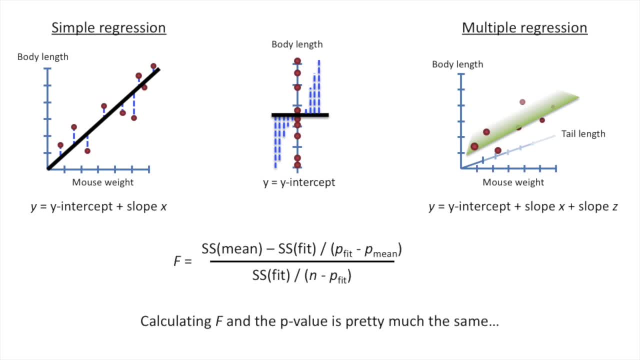 for linear regression, so it's no big deal. Now we want to calculate a p-value for our r-squared. Calculating f and the p-value is pretty much the same. You plug in the sums of squares around the fit and then you plug in the sums of squares around the mean For simple. 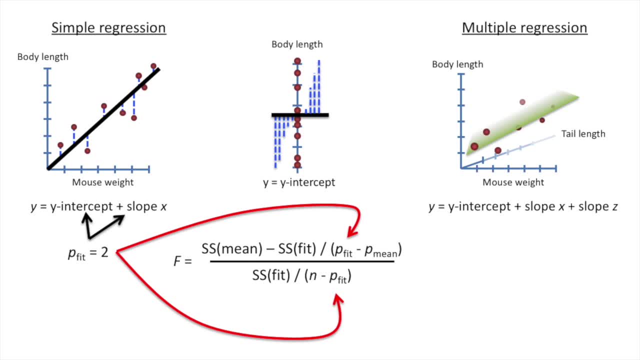 regression, p-fit equals two because we have two parameters in the equation that least squares has to estimate And, for this specific example, the multiple regression version of p-fit equals three because least squares had to estimate three different parameters. If we added additional data to the model, for example the amount of time a mouse spends, 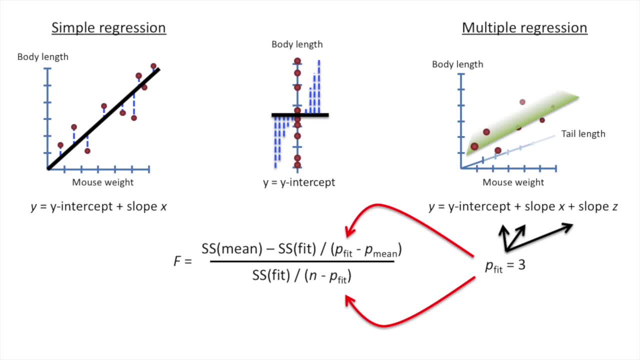 running on a wheel. then we have to change p-fit to equal the number of parameters in our new equation And for both simple regression and multiple regression p-mean equals one, because we only have to estimate the mean value of the body length. So far we have compared this simple regression to the mean and this multiple regression. 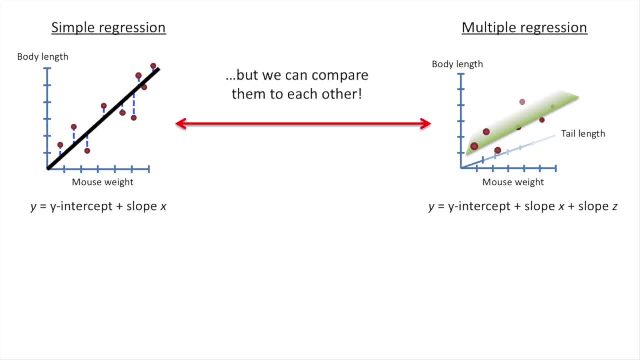 to the mean, But we can compare them to each other, and this is where multiple regression really starts to shine. This will tell us if it's worth the time and trouble to collect the tail length data, because we will compare a fit without it, the simple regression, to a fit with. 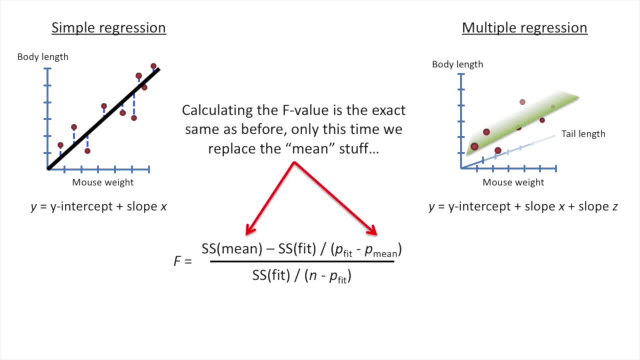 it. the multiple regression Calculating the f-value is the exact same as before, only this time we replace the mean stuff with the simple regression stuff. So instead of plugging in the sums of squares around the mean, we plug in the sums of squares around the simple regression. And instead of plugging in p-mean, we plug in.